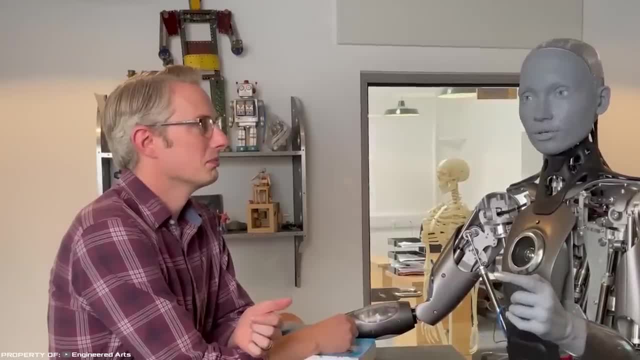 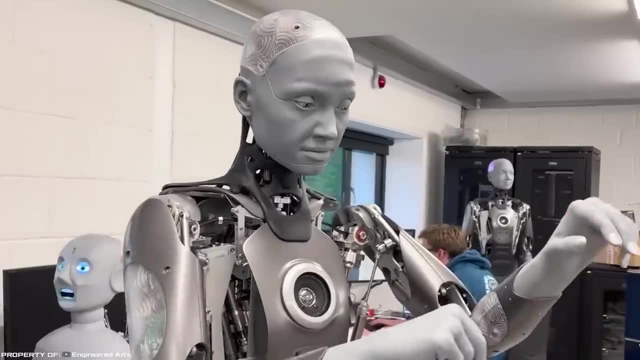 second generation of Amica, which has become even more realistic. This was achieved by increasing the number of motors throughout the head, the jaw, eyeballs, eyelids, eyebrows and even in the nose. Despite all these advancements, the robot still cannot walk. Therefore, 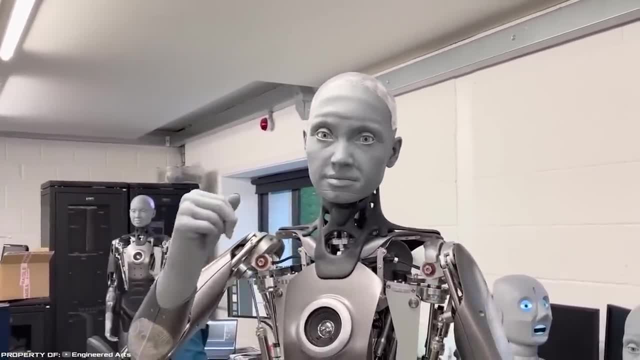 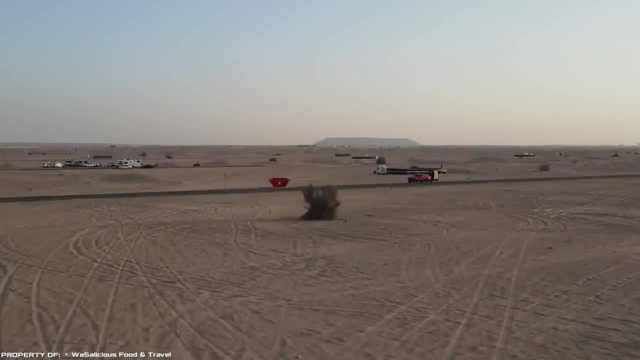 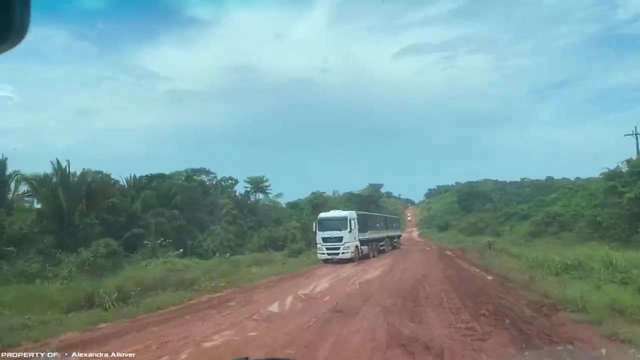 people who are afraid of a robot uprising can still sleep soundly for some time. 4. WaterGen- Mobility. Obtaining drinking water while traveling is not an easy task, especially if your route passes through the desert or areas where tap water is unsafe or unavailable. Now, thanks to the 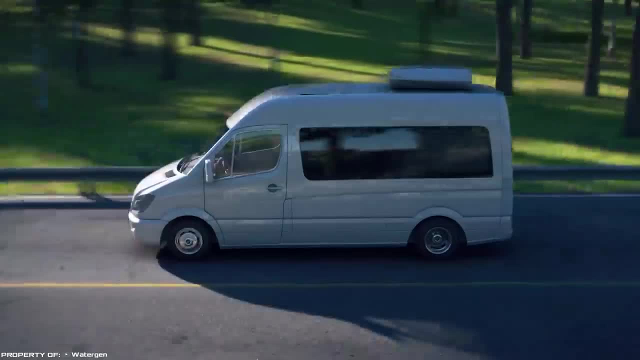 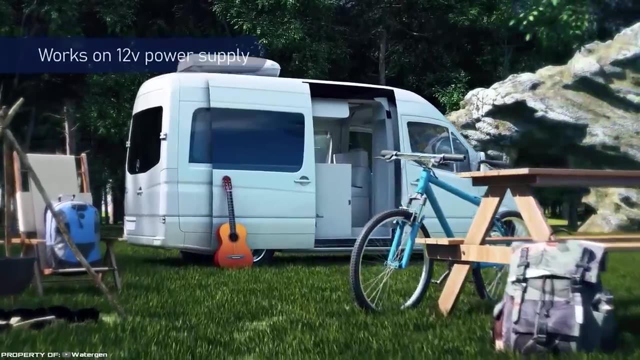 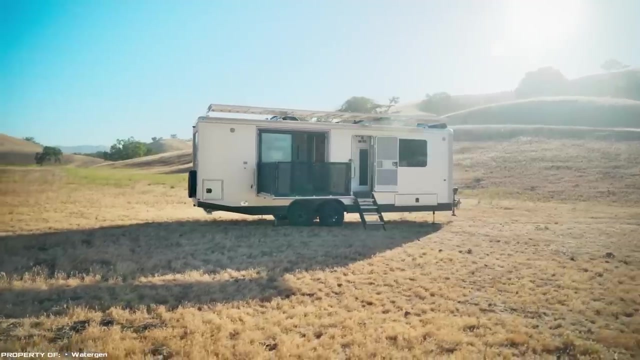 WaterGen Mobility unit. this vital liquid for the human body can be extracted from the air. The device developed by the Israeli company with the same name resembles a regular portable generator. However, instead of generating electricity, the device extracts water from the atmospheric air. Using a fan, the unit sucks in air from the environment and pumps it through. 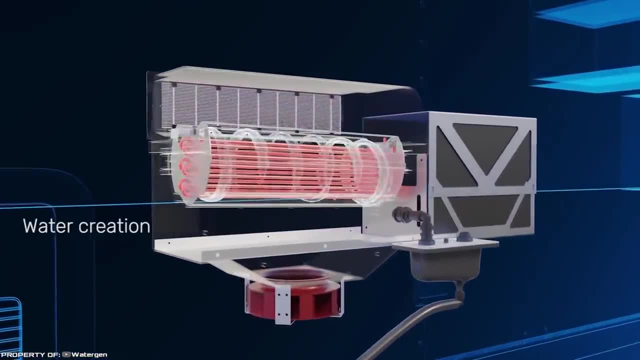 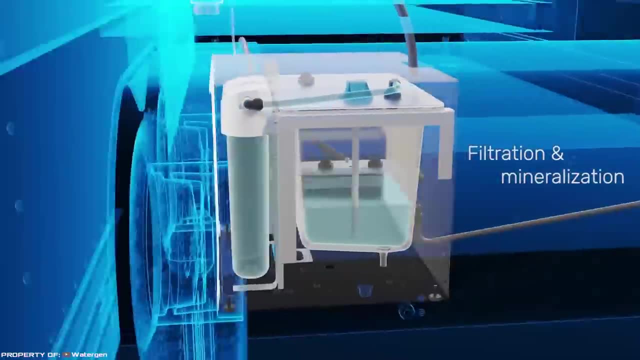 a patented heat exchanger system which extracts liquid in the form of condensate. The collected water passes through a multi-level filtration system and is collected in a special tank. The productivity of such an installation is up to 5,000 gallons. 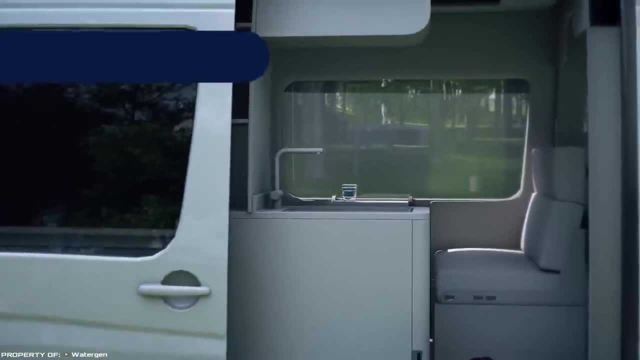 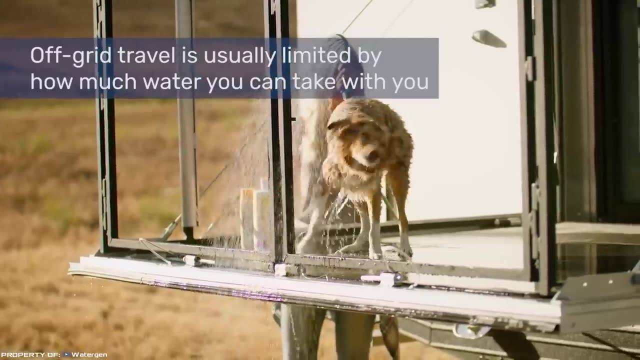 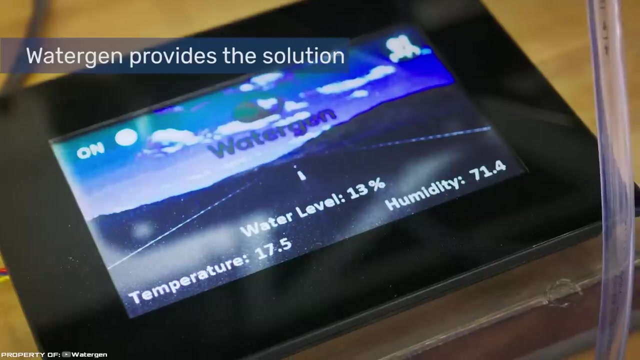 The device works from a 12-volt car socket or a standard 220-volt socket. The company living vehicle went even further and developed a highly autonomous camper that is capable of providing its inhabitants with both electricity and drinking water. The equipment for generating water from the atmosphere and other electronic devices of the trailer work. 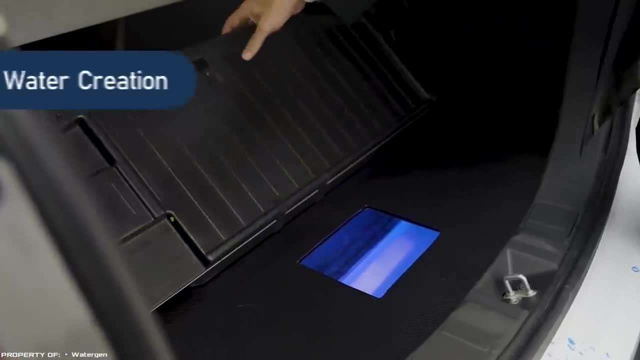 from solar panels. The water production capacity of the unit is about 5 gallons a day, which is enough to feel comfortable even if the tank is full of water. The unit is also equipped with a water pump and a water pump. The unit is also equipped with a water pump and a water pump. 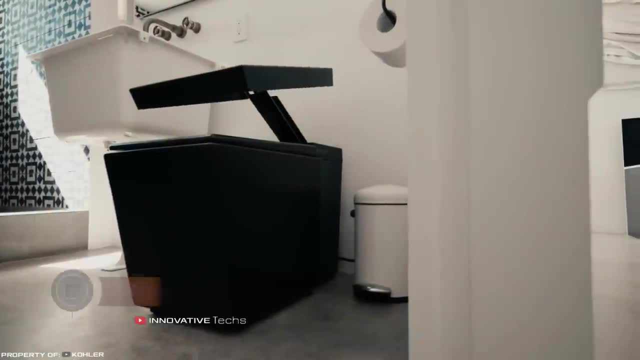 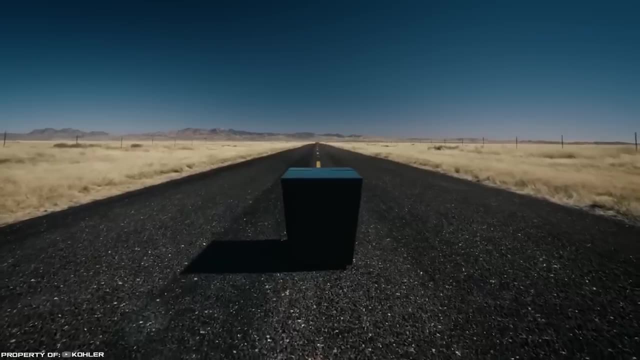 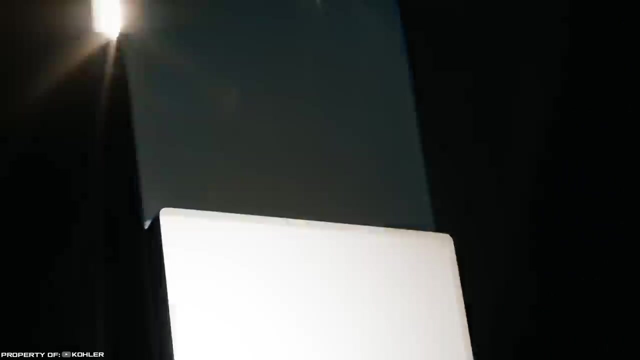 The unit is also equipped with a water pump and a water pump. Kohler Numi Smart homes no longer surprise anyone, but a smart toilet is something new. At the end of last year, the American company Kohler presented its novelty, the Numi 2.0 Smart. Toilet with the Amazon Alexa Voice Assistant, which allows you to control the functions of the plumbing fixture with voice commands. Numi 2.0 can greet the owner automatically, raising or lowering the temperature of the toilet and seat with heating. In addition, the novelty has an 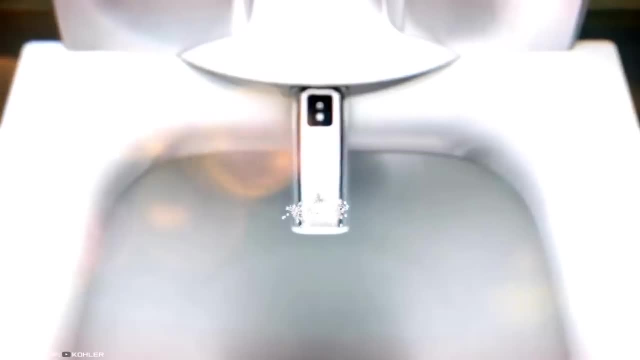 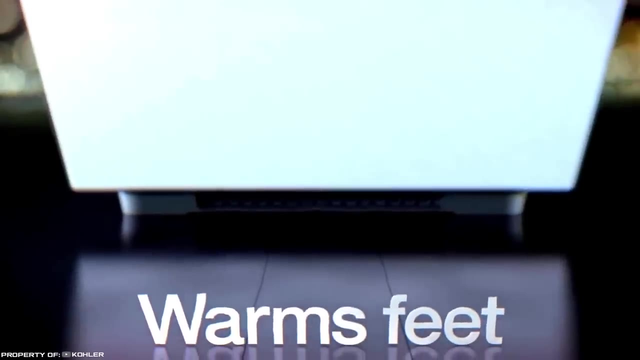 automatic flush and bidet function, with the ability to adjust the temperature, pressure and angle of the water stream. The toilet is also equipped with a system for supplying warm air to the feet, an emergency flush function, deodorization and air freshening. 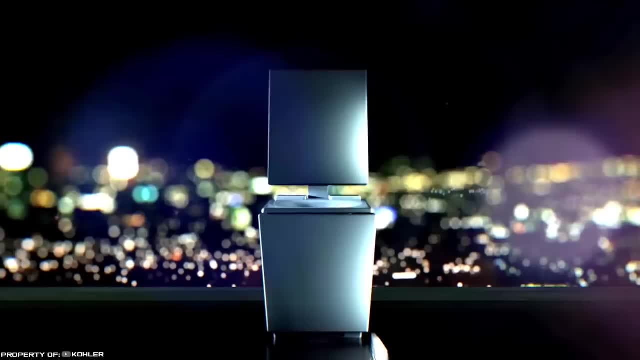 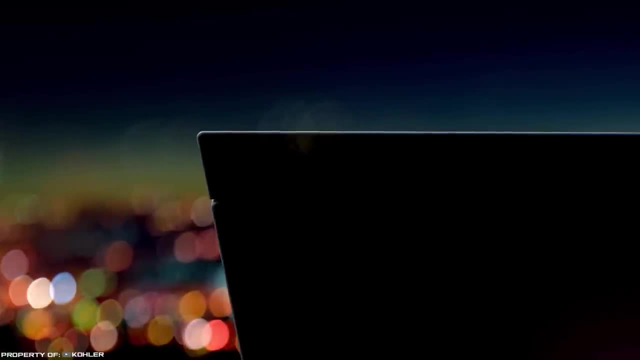 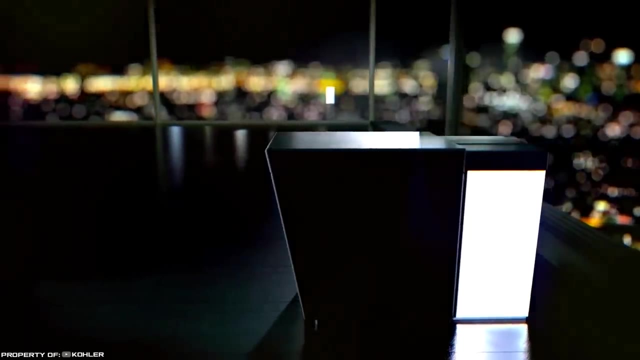 But that's not all. The device is equipped with speakers that provide rich stereo sound, helping to hide unwanted noise or relax in the bath to favorite compositions. The cost of the novelty corresponds to its intelligence and is $11,500.. Smart Thermometer Meter. 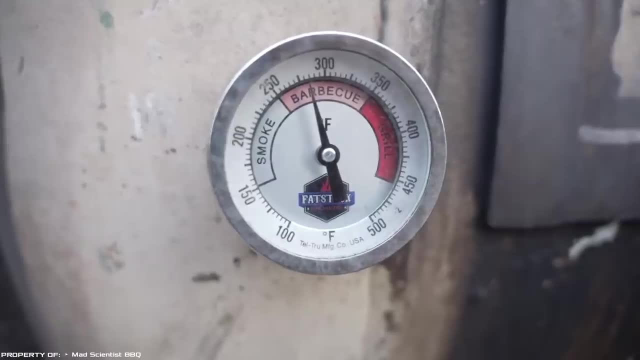 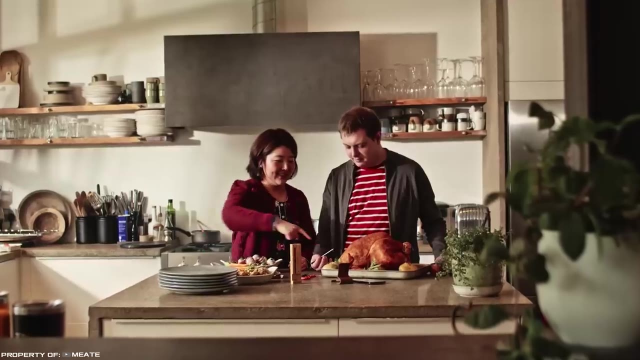 We all love to eat delicious food, especially meat, But how do we ensure the proper temperature regime of its preparation without experience? Meter comes to the rescue, a wireless thermometer that allows remote monitoring of the degree of cooking of steaks and other meat dishes. 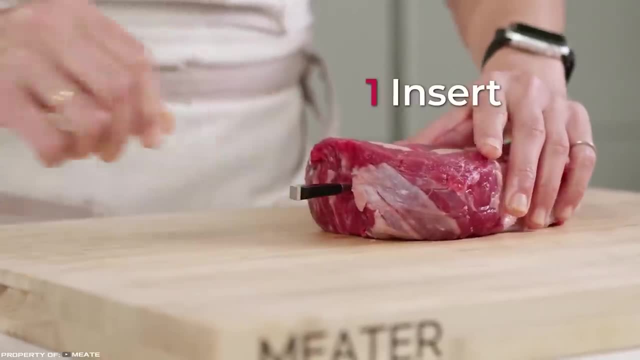 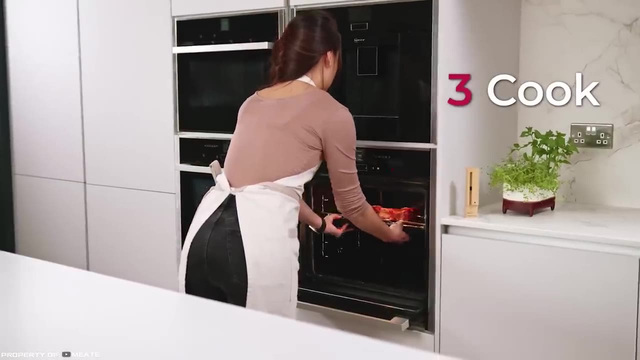 The device has a built-in Bluetooth and Wi-Fi module. The device has a built-in Bluetooth and Wi-Fi module. Using the thermometer is easy. The app offers the option to choose a recipe, type of meat- chicken, beef, pork- and the degree of its roasting. 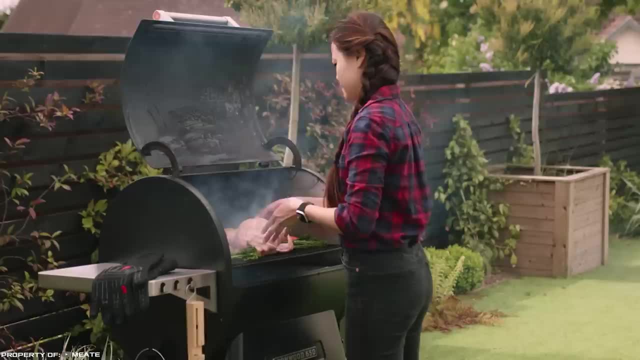 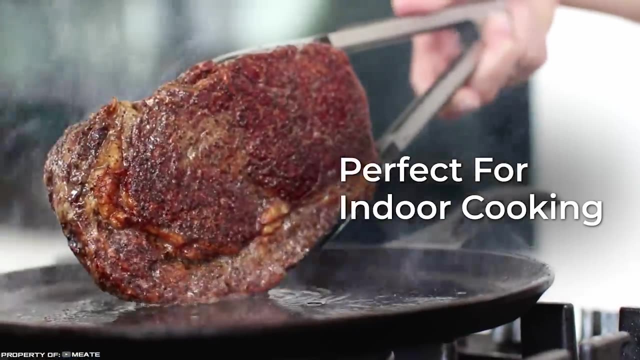 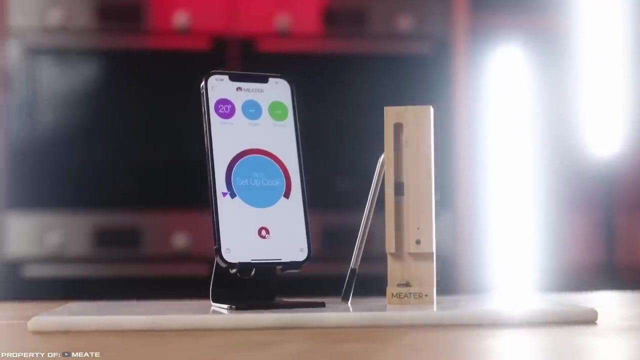 Then meter is inserted into the meat, which is then sent to the grill or oven. A special app allows you to monitor the cooking process in real time and sends a notification to your smartphone when the dish reaches the desired roasting level: rare, medium-rare or well-done. The device is powered by a built-in battery. 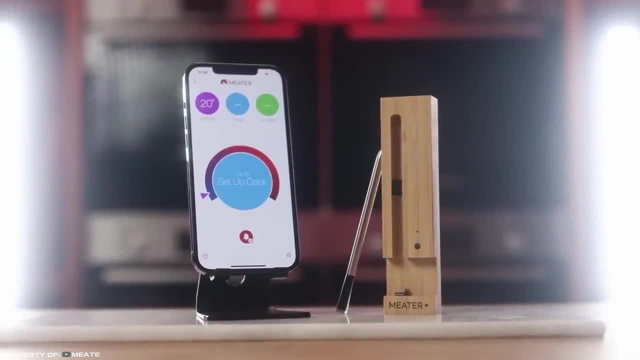 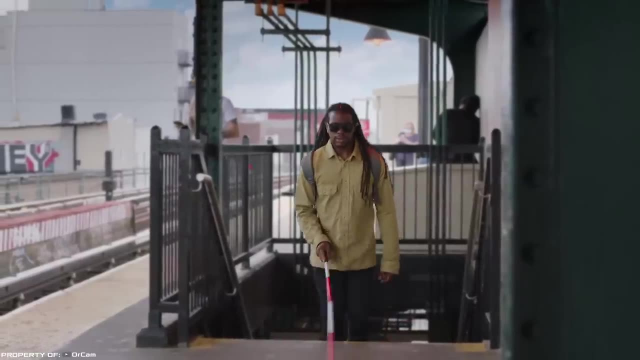 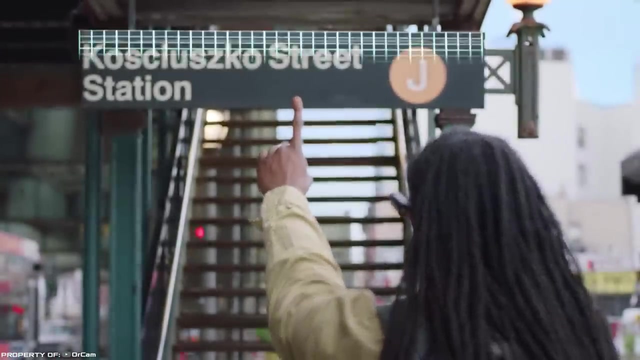 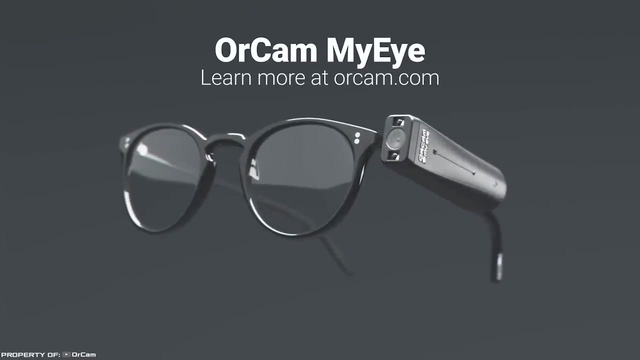 which lasts for 24 hours of continuous operation. MyEye Pro. Millions of people around the world have limited ability to see the world around them. For them, OrCam has developed smart glasses that help them read printed and digital text, recognize people or identify objects. We are talking about the MyEye Pro device. 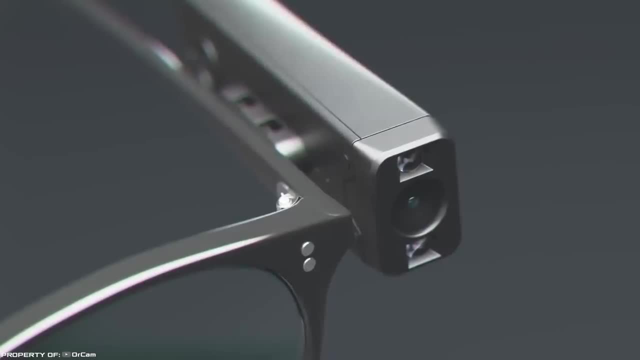 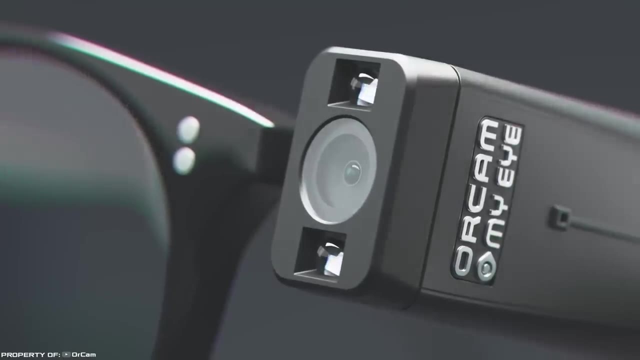 which transmits visual information in an audio format. To use it, you need to attach the device to the frame of ordinary glasses, using magnets To activate the ability to recognize faces or to make it read pages in books, newspapers or menus in a restaurant. 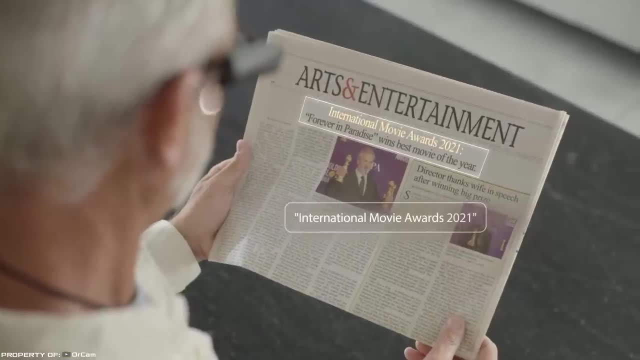 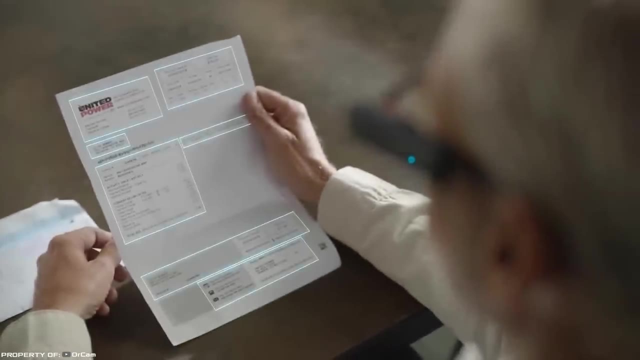 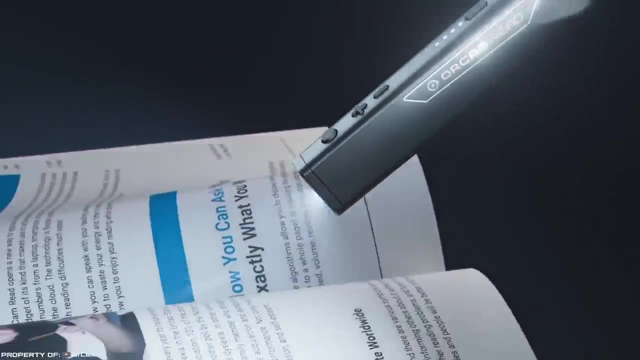 you need to ask the voice assistant. For example, you can ask the gadget to read the headlines in the newspaper and then voice the interesting article. In addition, the device quickly and accurately responds to pointing gestures, identifies barcodes and banknotes. MyEye Pro is equipped with a fast processor, two microphones. 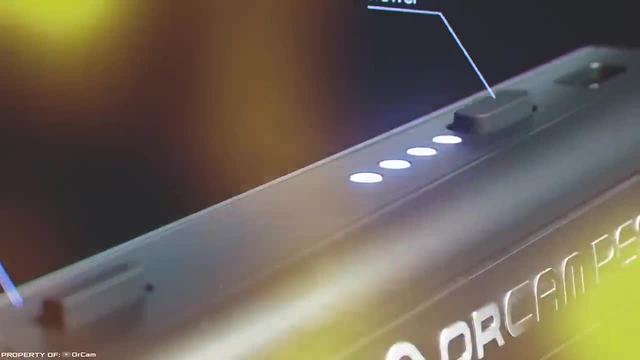 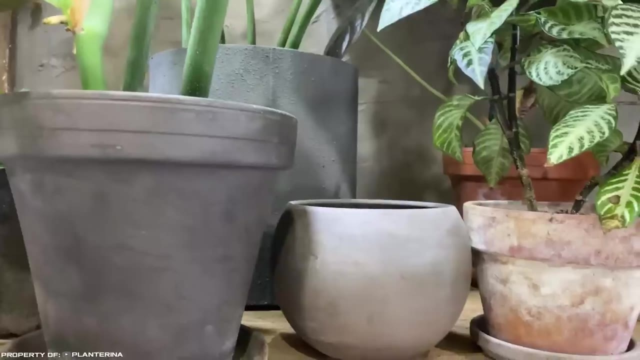 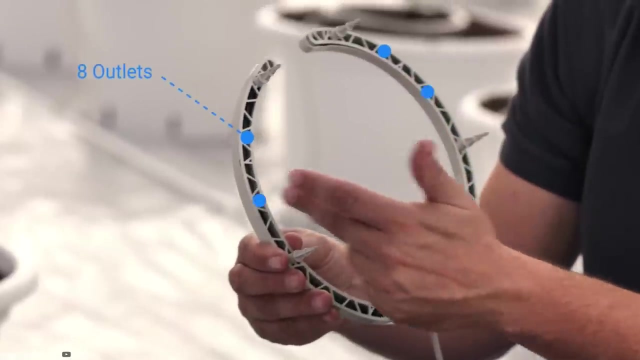 and has a long-lasting battery life. Netbo: Plant lovers who grow plants in pots know how difficult it is to provide even watering for the entire root system. Now this problem is solved. The Israeli company Netafim has presented a unique Netbo drip irrigation system that ensures complete, uniform distribution. 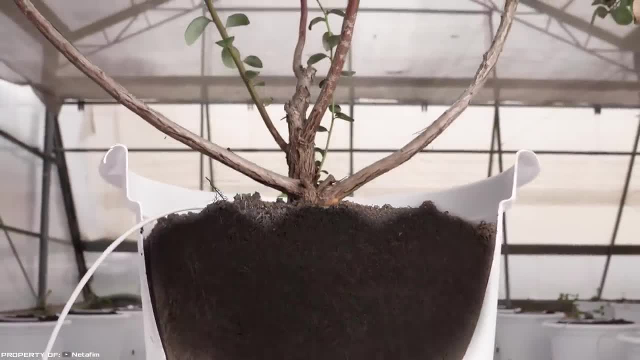 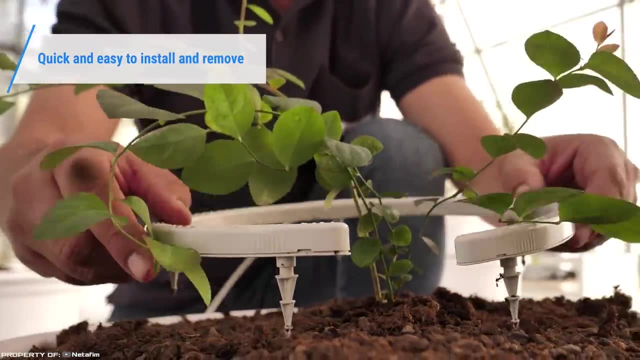 of water and nutrients throughout the root system for even growth. The device is small in size, with eight typhoon drippers that are highly resistant to clogging, and it is easy to connect and install. The Netbo system was specifically developed for growing valuable soilless crops such as: 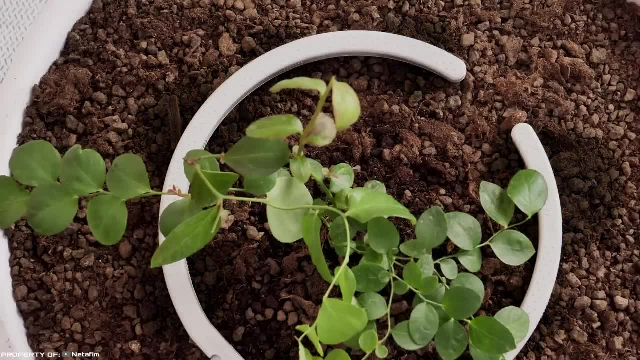 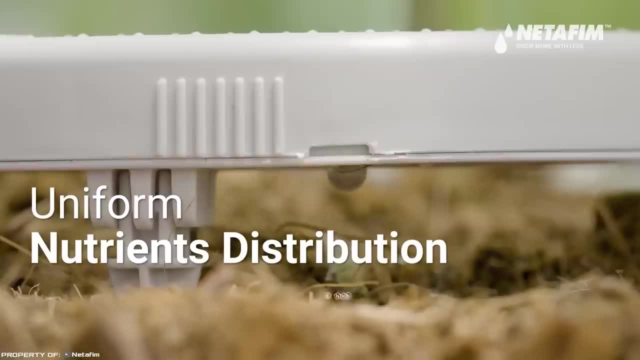 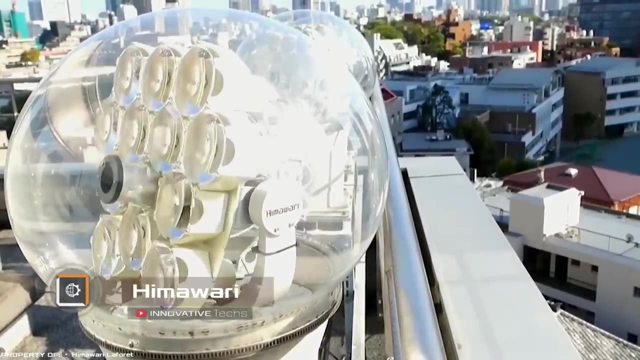 blueberries and cannabis, which require special irrigation and fertigation technologies. By using such a device, the roots develop on every square inch of the container, including the top layer, where it is especially important: Himawari Solar. Many people are familiar with the situation when a neighboring house is located too close. 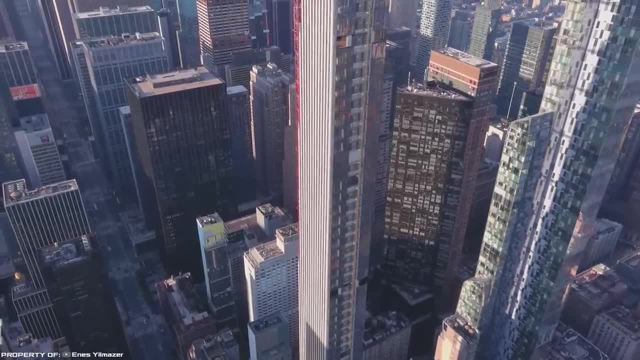 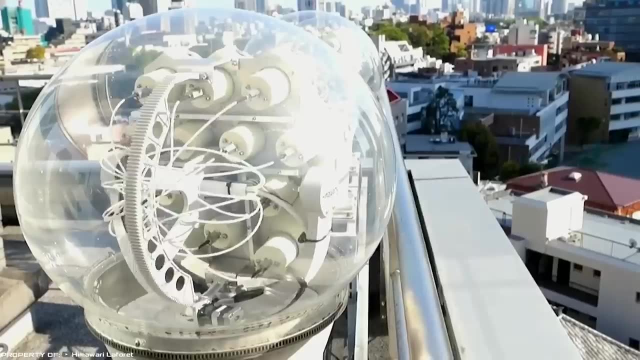 to a large tree that prevents sunlight from entering a room. Workers in warehouses, production workshops and offices also often face a lack of proper natural lighting. The Himawari system can help solve this problem. The device is a complex of lenses that collect. 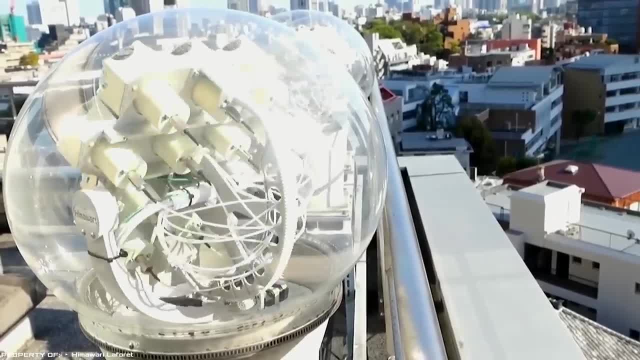 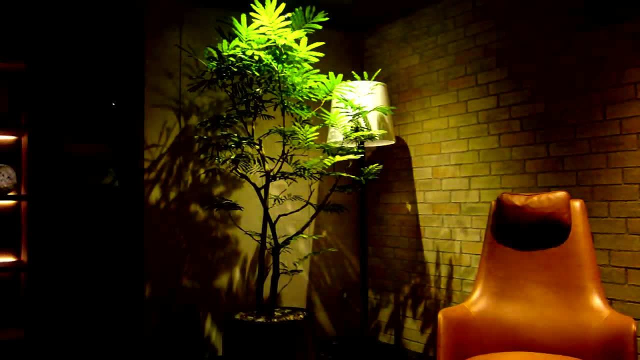 sunlight and transmit it through optical fiber cables to a lighting element located in the room. Thanks to this innovation, it is possible to not only provide a home or office, but also provide a home or office with full natural lighting, but also to save on electricity bills. 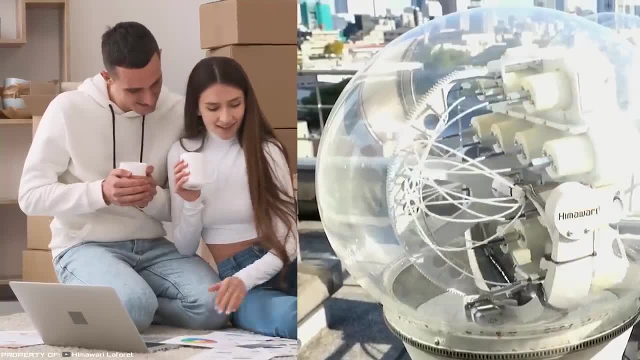 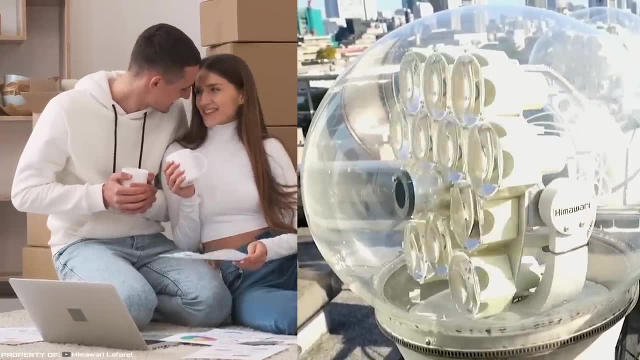 And that's not all. The Himawari Solar device is equipped with an automatic tracking system that accurately determines the direction of the sun's rays and constantly changes its position. The presence of such a function allows natural lighting in the room throughout the day. 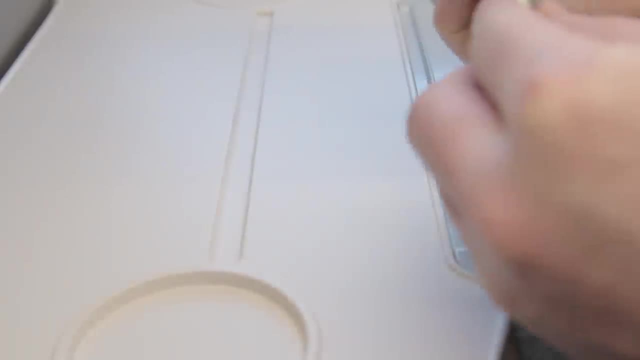 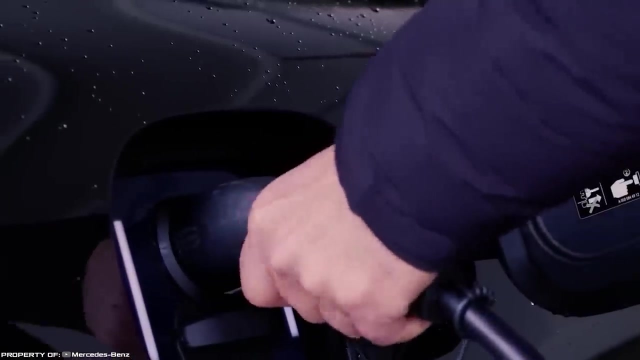 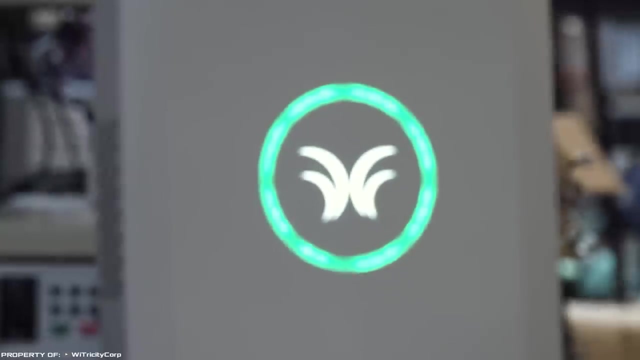 WeTricity. You probably know that the most annoying problem with smartphones is the need for regular charging with a cable. Owners of electric cars face a similar problem when they need to refuel their vehicle. However, in the near future, everything may change drastically. WeTricity has announced a partnership with General Motors to test the latest wireless 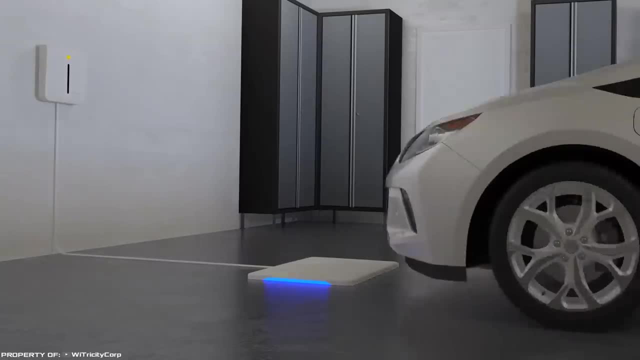 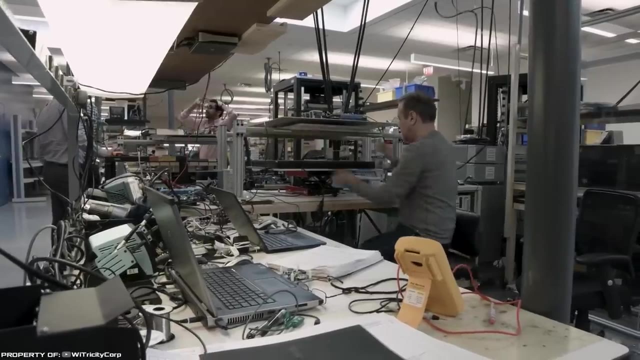 charging system for electric vehicles. WeTricity's technology is based on the magnetic resonance effect and involves the use of electromagnetic waves. The new device consists of a receiver and a transmitter of electricity. The first wave of electromagnetic waves is the first wave of electromagnetic waves. The new device consists of a receiver and a transmitter of. 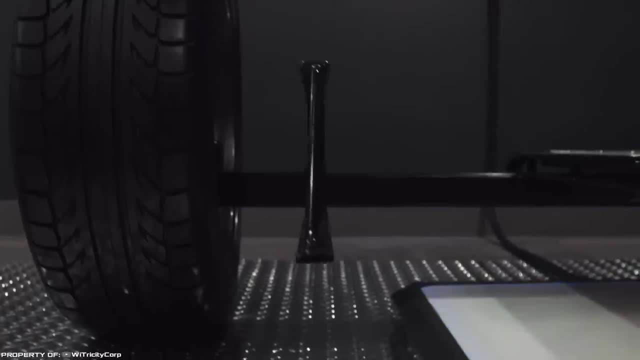 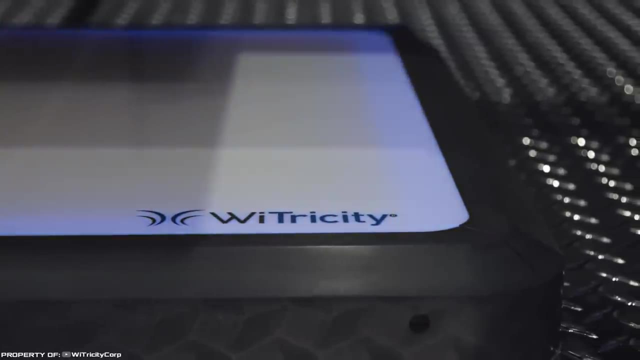 electricity. The first one is installed in the electric car and the transmitter is located in the parking area of the vehicle. The ground clearance of serviced electric cars can vary from four to ten inches. The prototypes that WeTricity and GM plan to test provide power. 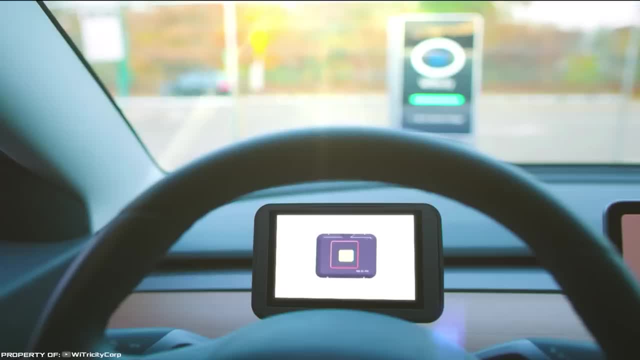 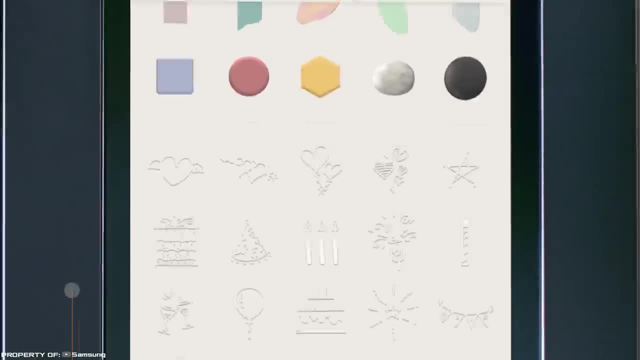 of 7 kilowatts and 11 kilowatts and will be used for wireless charging of both fully electric vehicles and hybrids. Samsung Family Hub. Samsung Family Hub's myself has been ahead of its time by introducing a new model and its own device. 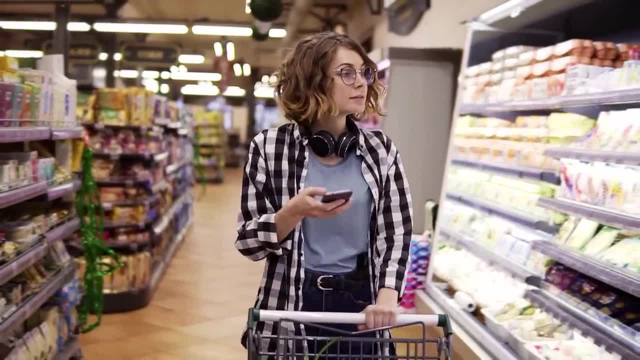 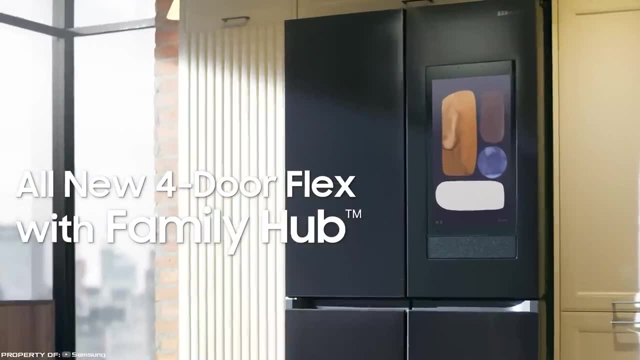 Constantly forgetting what products to buy at the store or not knowing what to cook for dinner? Then the Samsung Family Hub Refrigerator with AI is made just for you. The gadget is equipped with cameras and takes photos of its contents every time the door is closed. 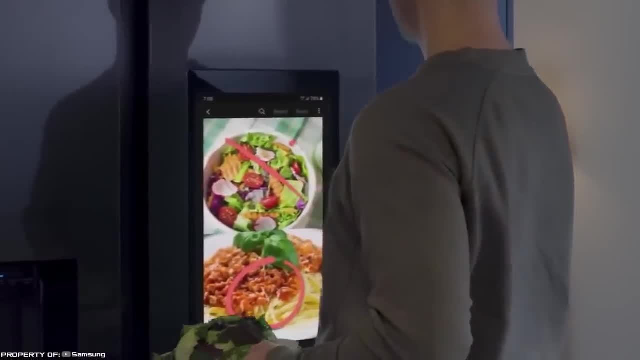 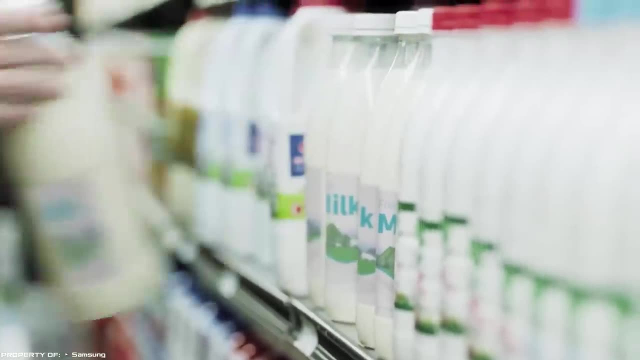 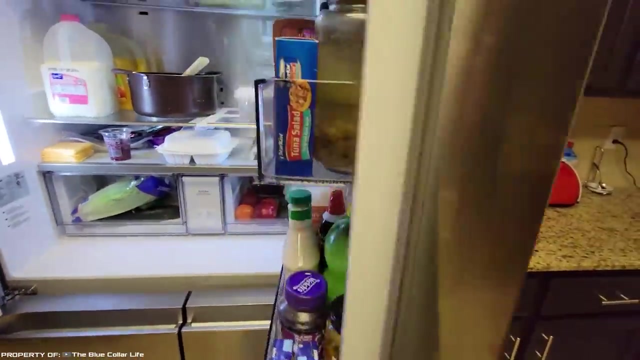 These images are uploaded to the cloud, allowing you to view them from your smartphone. Therefore, if you find yourself in a store and can't remember what else you need to buy, you can always access your food supplies. In addition, the built-in AI in the device plans your diet for up to a week and automatically. 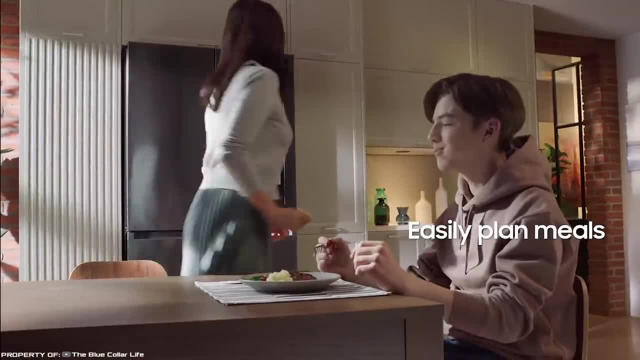 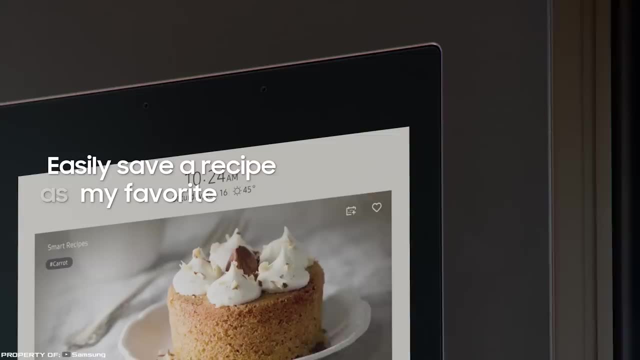 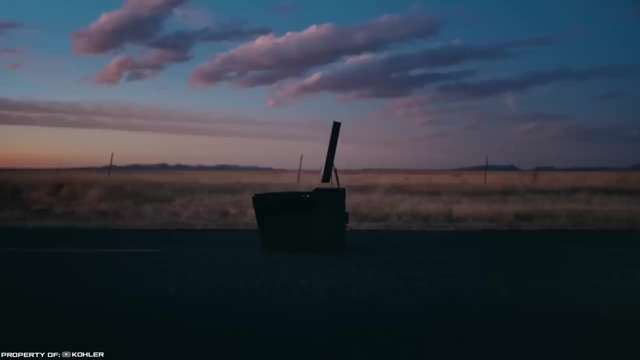 creates a shopping list of ingredients that can be used to prepare several dishes at once. It is likely that the Samsung Family Hub is just a concept. However. the rapid development of AI technology suggests that such refrigerators may soon become available for purchase. What other inventions do you think could make our lives even more comfortable? 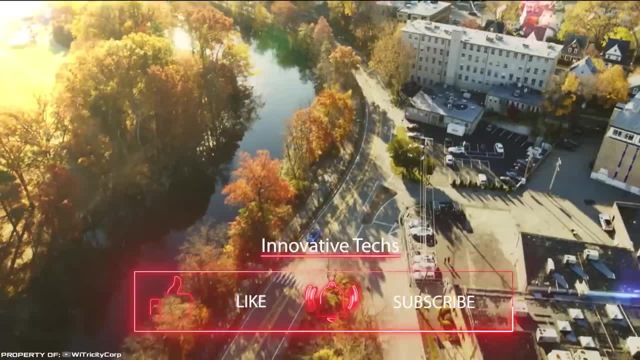 Share your thoughts in the comments and don't forget to subscribe to our channel. There are still many interesting facts from the world of science and technology.